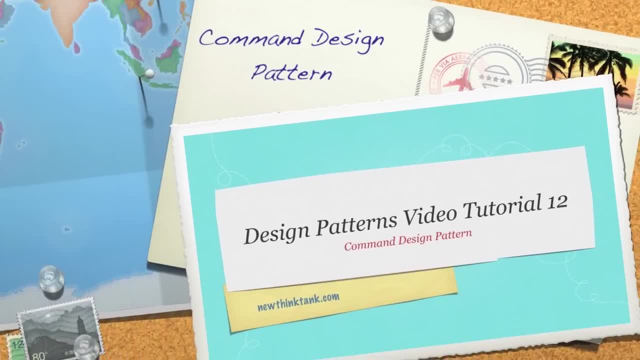 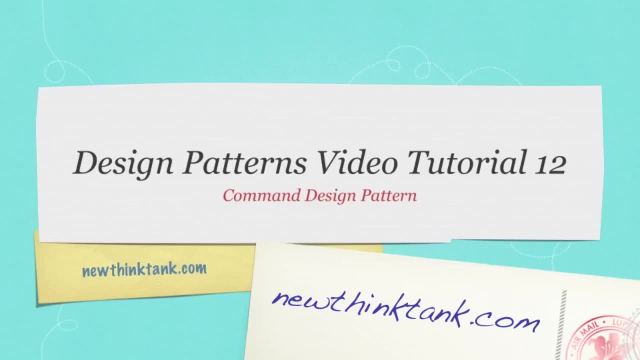 Well, hello internet and welcome to part 12 of my design patterns video tutorial. Today we're going to talk about the command design pattern. I'm going to show you this in numerous different ways. I'm going to explain it as a simple definition. I'm going to explain it as a walkthrough, just using words. Then I'm going to show you a UML diagram, Then, on top of that, I'm going to show you all of the code, And then, on top of that, all the code is available underneath the video. So if you go through all five or six of those steps, I guarantee you will understand the command design pattern. So let's get into it. So what is the command design pattern? Well, the basic. 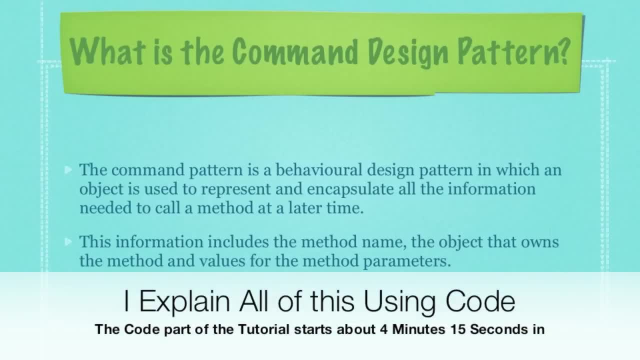 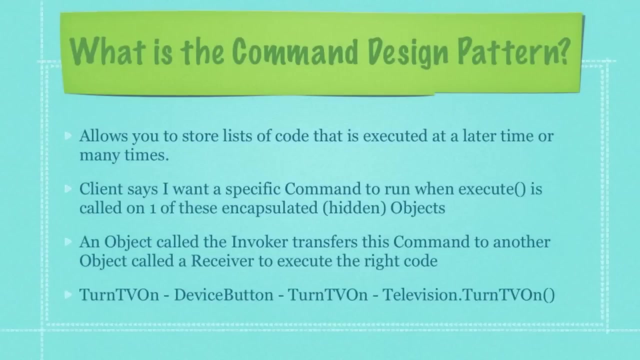 definition is: the command design pattern is a behavioral design pattern in which an object is used to represent and encapsulate all the information needed to call a method at a later time. This information includes the method name, the object that owns the method and the values for the method parameters. Now, if that didn't make any sense, let's move on and explain it in a completely different way. Basically, what it allows you to do is store lists of codes that are executed at a later time or many times, And on top of that, normally with the command design pattern, there is a capability for you to undo. 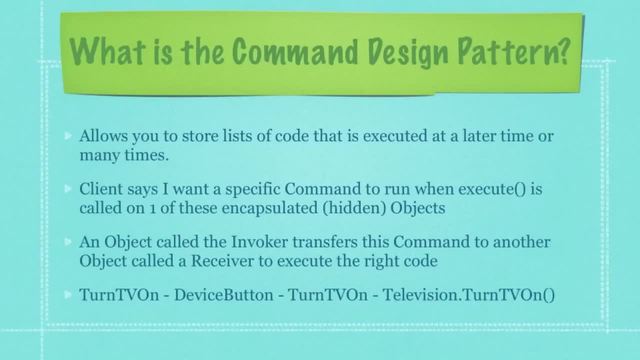 commands. Basically, what happens is the client or the application part of your program says: I want a specific command or a list of code to be executed whenever a method called execute is called on one of these encapsulated hidden objects, And then an object called the invoker, whenever it is invoked to perform a command to set it in motion, transfers this command to another object that is called the receiver, and the receiver has the actual code that you want to execute and whenever it 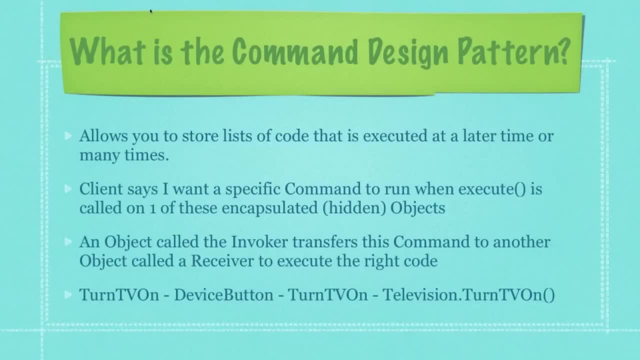 gets the command from the invoker to execute it, it executes it. So, basically, if we have this object down here called turn TV on, this is actually a command. This command is defined, then device button, which is another class or object that's going to be created. whenever it is called, it sends turn TV on. Of course there's going to be interfaces between all this so we can use polymorphism. So whenever turn TV on is called, that method then will be executed by the receiver. 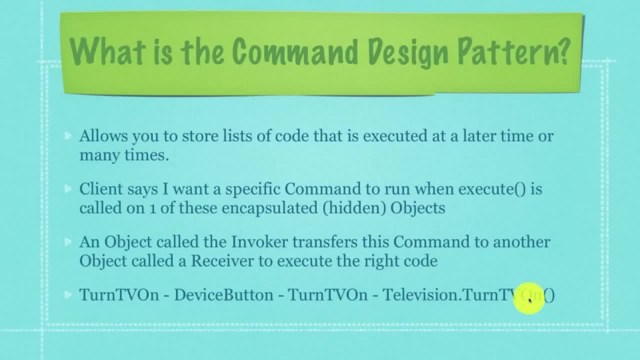 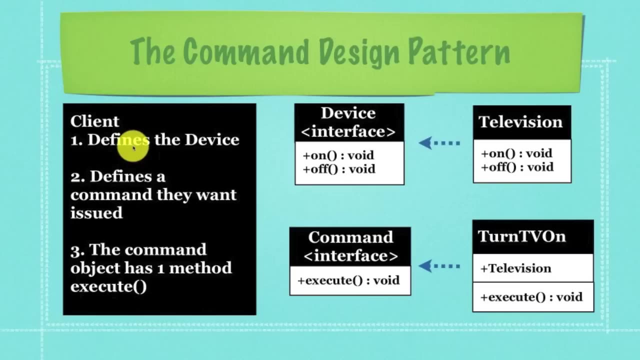 Or television, another object, and here is turn TV on. So there's another explanation. So let's look at it from another way. OK, Here is the client again, and it's going to define a device which is going to be an object that's going to contain a whole bunch of different methods that can be run for that very specific device object. It's going to define a command that they want to be issued. This is again the application part of the client, and the command object has one method inside of it called execute. You can see everything over here, So let's 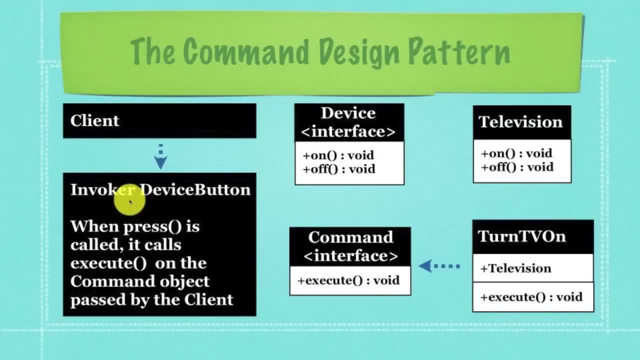 bring in the invoker to this and then explain everything that goes on. OK, Here is the invoker, which is just going to be an object that is going to have a method inside of it. In this situation it's going to be called press. Now, when press is called, it's going to call execute on the command object. Here is execute as I am referring to it. Of course, it's going to refer to it through an interface for polymorphism, But either way. So press is called on this object called device button and it calls execute on turn TV on. 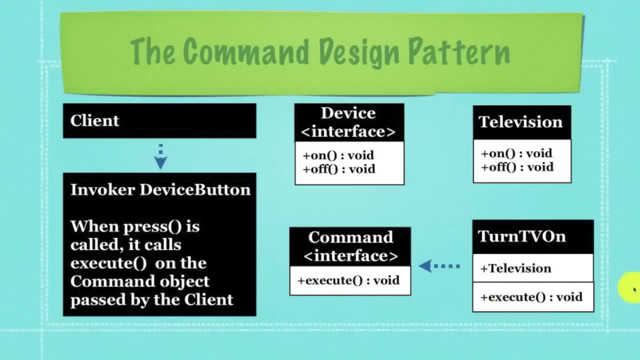 Then what happens is execute tells the television object that is right here to execute the on method which is up here in this television object, In essence that is the command design pattern Device button is called, specifically press a method inside of it- or at least that's what I'm going to use- Then execute is called on a another object called the command object. Execute is over here. Whenever execute is called, all it does is it says: 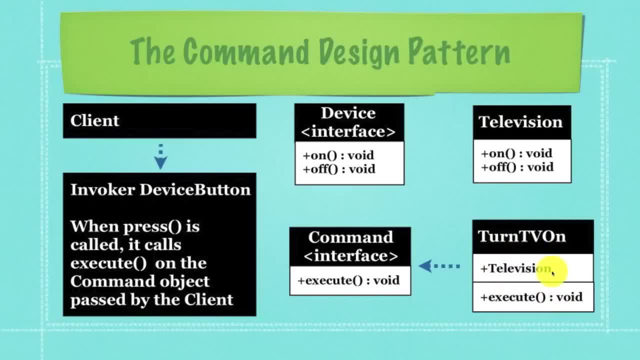 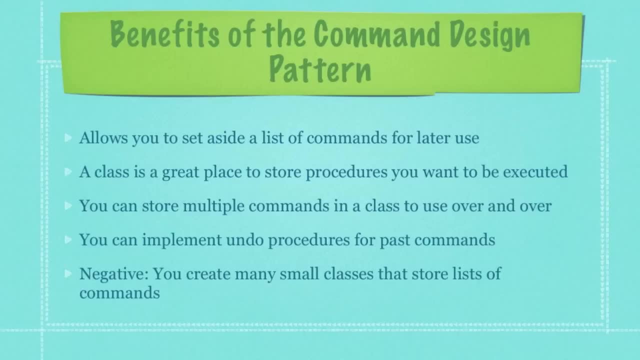 hey, my job as an object is to turn televisions on, So what I'm going to do is I'm going to tell the television object to execute the method on that is inside of it. So that's sort of an explanation in that regards. So what are the benefits of the command design pattern? Well, it allows you to set aside a list of commands for later use, Like I mentioned before. On top of that, a class is a great place to store procedures that you want to be able to execute multiple times. You're going to be able to store multiple commands in a class to use over and over And on top of that, like I said before, multiple 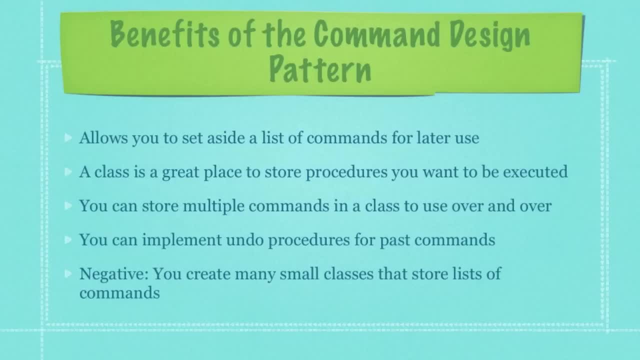 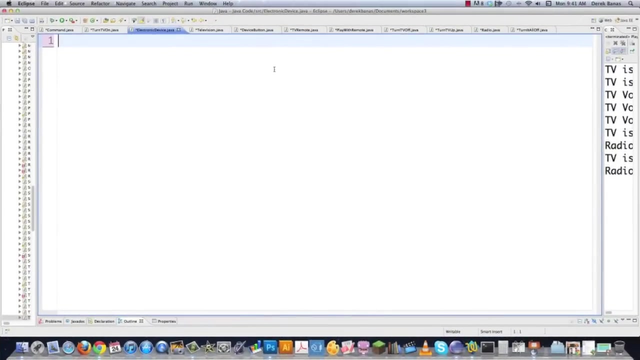 Most of the time, you're going to implement undo procedures so that you can undo previous commands. The only negative with the command design pattern is that you need to create many small classes to store lists of these commands. So that's a basic rundown, So let's just jump right into the code. All right, So the first thing that I'm going to need to do here is to create an interface that is going to be used to create all of my receivers. That sounds really complicated, but it's really not. So I'm going to create an interface and it's going to be called electronic device And basically what I'm 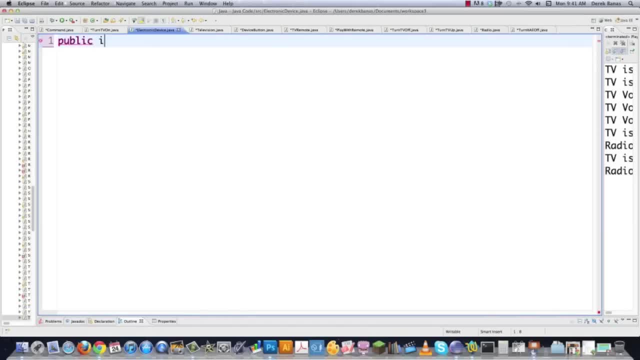 What I'm going to do is implement a remote control sort of system here. So real simple. we're just going to go: public interface, electronic device, okay, So there's going to be our interface that we're going to build all our receivers from. 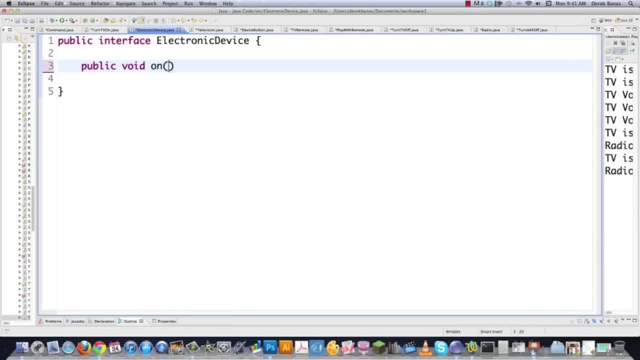 And then I need to define all of the different methods that each one of these devices is going to have, So on: it's going to be able to turn itself on, it's going to be able to turn itself off, it's going to have the capability to turn the volume up, and it's also going to have 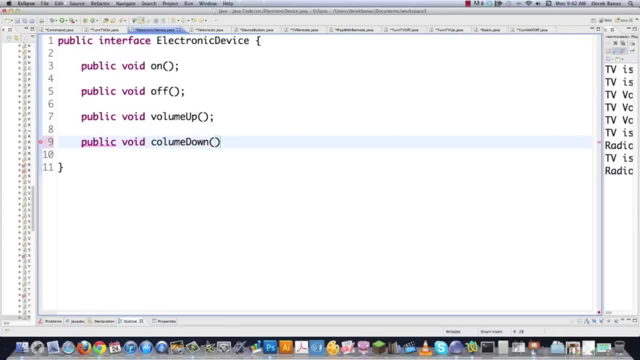 the capability to turn the volume down. And there you are. And, of course, make sure you spell it right. So there's our interface that we're going to use to make all of our electronic devices or receivers, And so let's just jump right into it and let's make a receiver called televisionjava. 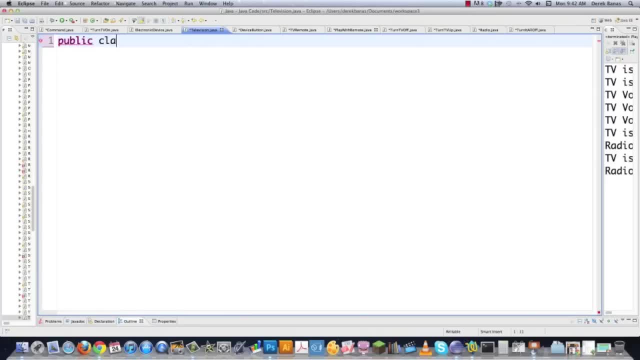 So here's televisionjava. We're just going to go public class television, And I know I say it all the time, but really, at least for myself, I wasn't able to completely understand this pattern until I saw it in print. 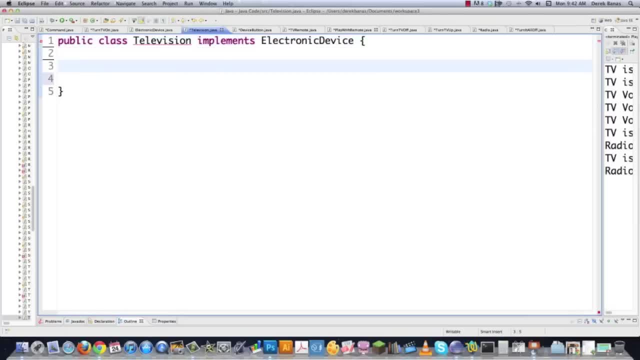 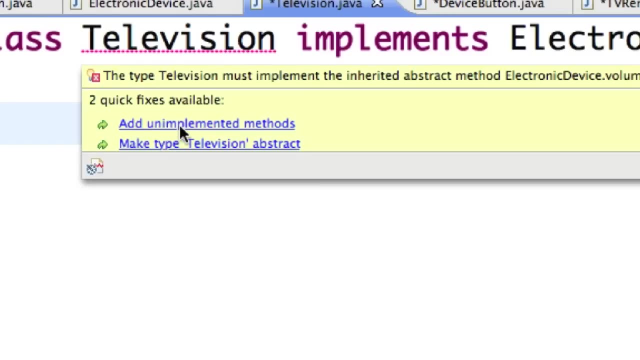 So of course I provide it. I do that option underneath this video. OK, so just going to implement that electronic device, And then we're going to come in here and Eclipse is going to allow us to add unimplemented methods, so I don't have to type all that stuff out. 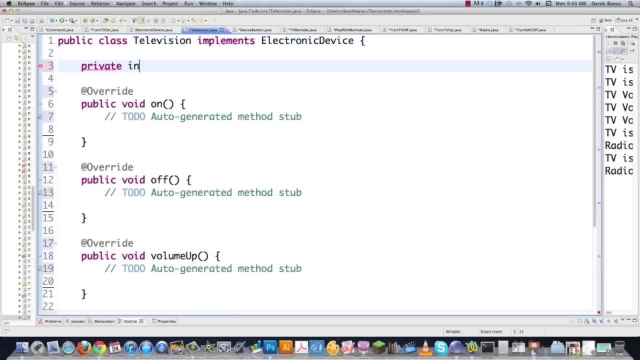 And then, inside of here, I'm going to create myself a private method And it's just going to contain a value for volume and it's going to start out at zero. And then I'm just going to keep this really simple. I'm going to say whenever these are called- of course you could have many different things- 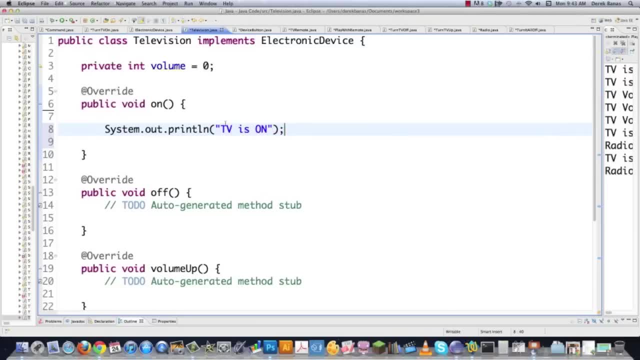 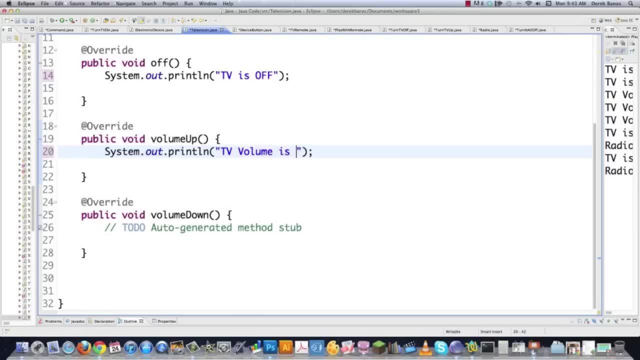 occur here. But I'm just going to say: TV is on, Just to keep it really nice and simple. And then in this situation, TV is off, TV volume is at, And then we'll just throw volume inside of there, which is that private variable that. 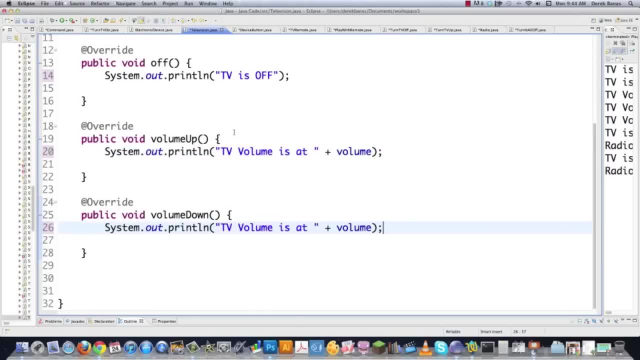 we have And TV volume is at, and throw that inside of there as well, And then all we're going to want to do here is just go volume plus, plus to increment that, And then volume, negative, negative. There you are. You just created yourself a receiver called television that's going to be able to implement. 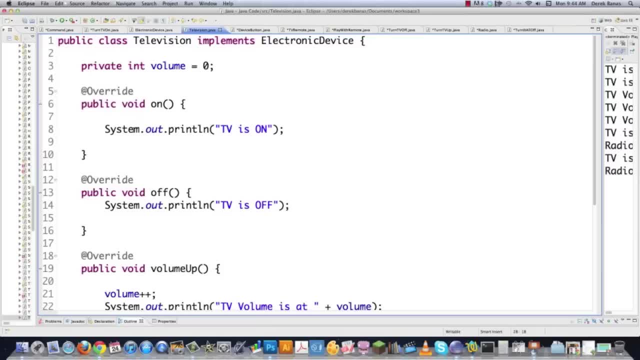 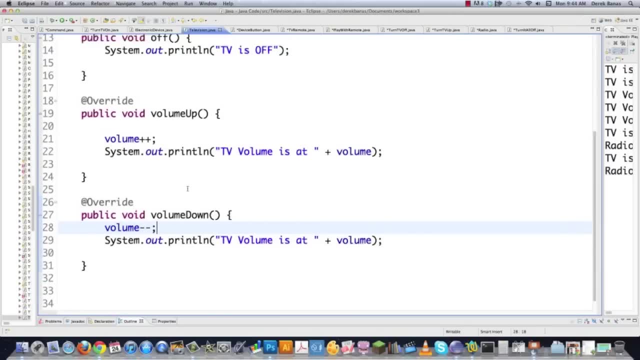 these very specific methods, And then you're going to want to go ahead and create a command that's going to be able to implement these very specific commands. Basically, all we're doing here is we're making commands very unspecific and eventually they will lead here to print and execute the actual real commands themselves. 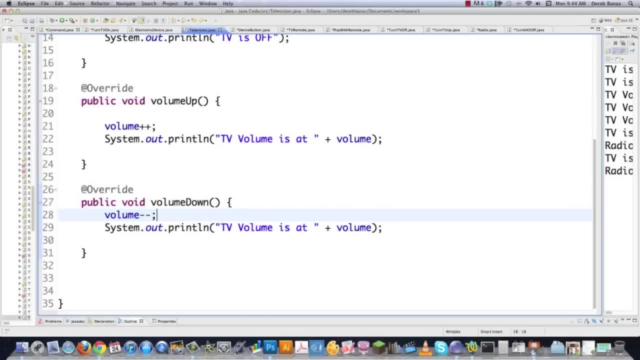 That's all you're going to have to do with that. So now let's go and create our command interface that every single command is going to have to implement, And it's going to be simple as well. We're just going to go: public interface command. 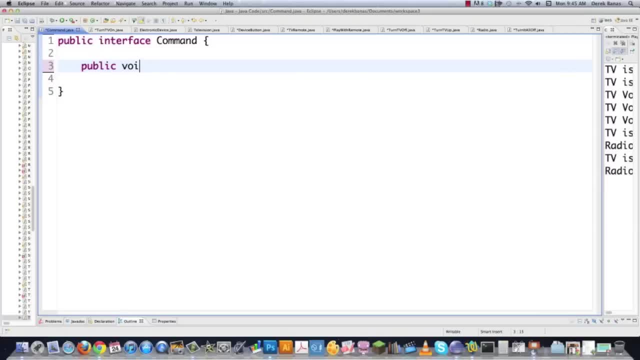 And this is going to be extremely simple. We're just going to say public void- execute. Anybody that wants to use this command interface must have an execute option. That's pretty simple, And guess what You're done. So now let's start creating some very specific commands. 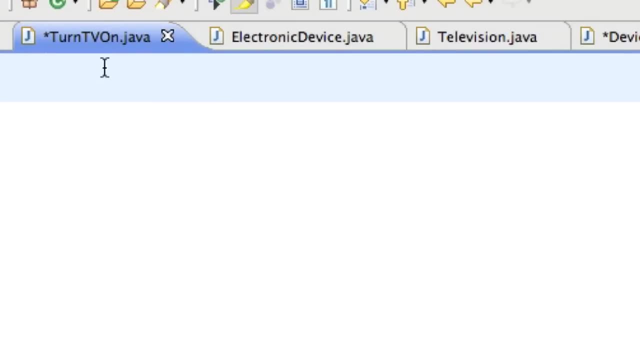 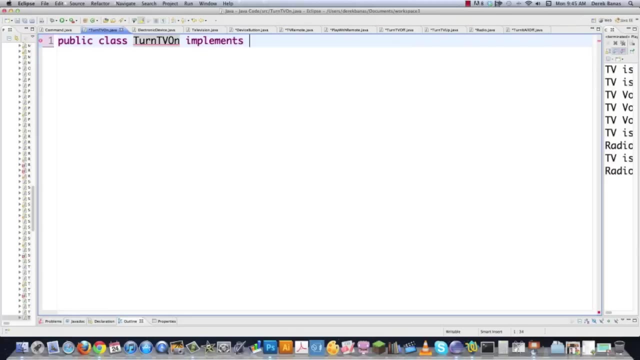 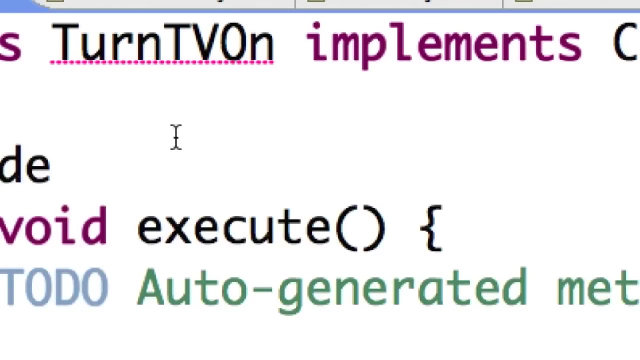 We're going to go into turntvonjava right there And we're going to go public class turntvon implements command, of course, because that's what we just created- And then have it come in here and put in my execute method so that everything is nice. 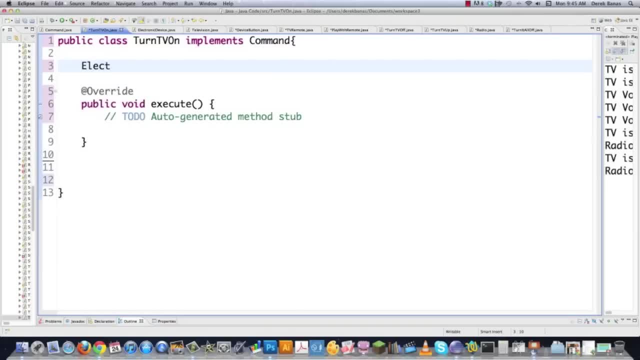 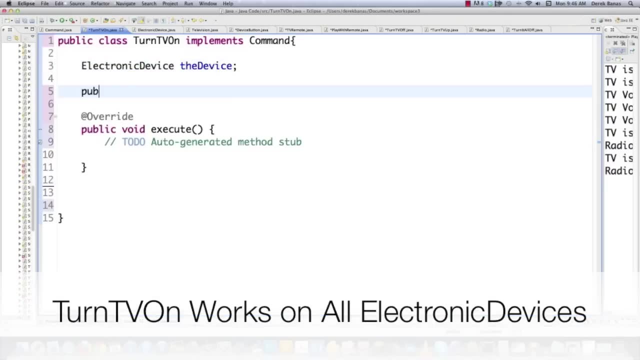 there, But this guy's going to need to know, OK, well, what exact electronic device do you want me to be working with? So I'm going to store that inside of here And then turntvon, I'm going to create a constructor here. 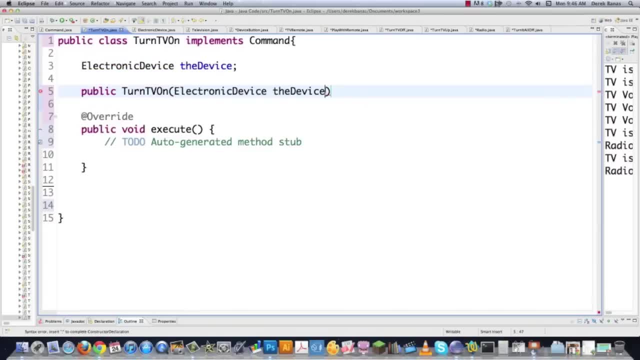 And it's just going to be passed an electronic device to perform this command on. except I'm going to change this to new device And then just go. the device is equal to new device, which is going to be passed to it. So very simple. 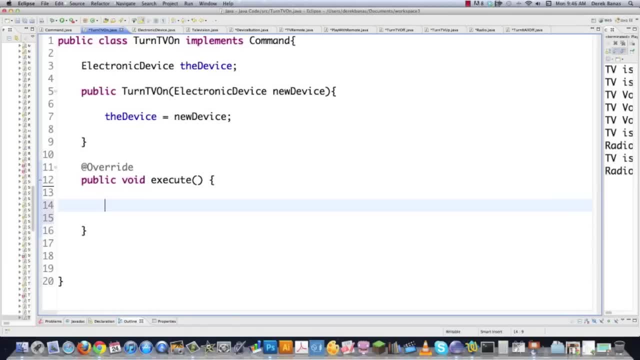 And then we come down to the execute part And it's going to say: OK, that device that you sent me, since I am known as the turntvon command. what I want to do here is call the on method for said device. 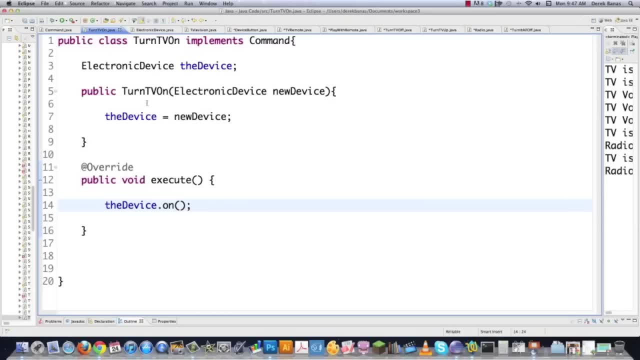 Boom, You're all done. That's all we need to do. You just implemented your first command object inside of here And guess what? Turntvoff is going to operate in much the same way. So where is turntvoff There? it is turntvoffjava. 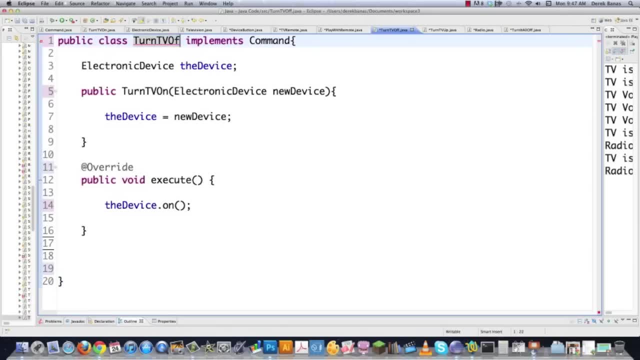 Click on that Paste inside of there- Turntvoff is going to be the name for that- And then we're just going to come through here and make a couple little changes, But pretty simple stuff. Just about everything is already done there. 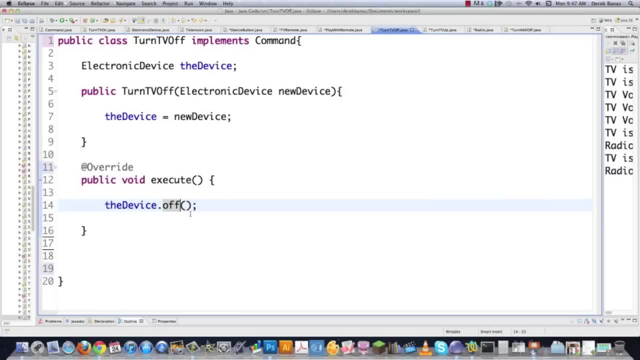 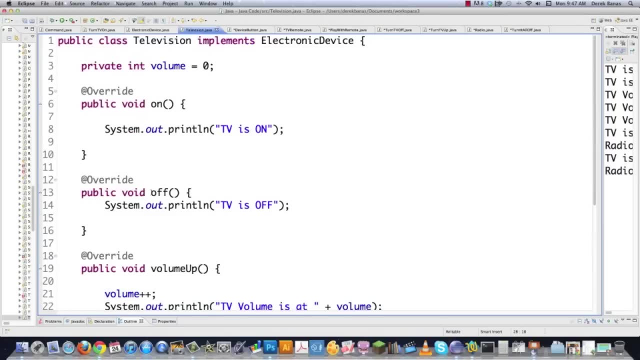 And then down here, since it's the turntvoff, we're going to call the off method on the device And, in case you forgot, let's just go over to televisionjava. All it's doing is coming here and calling these very specific methods for these very 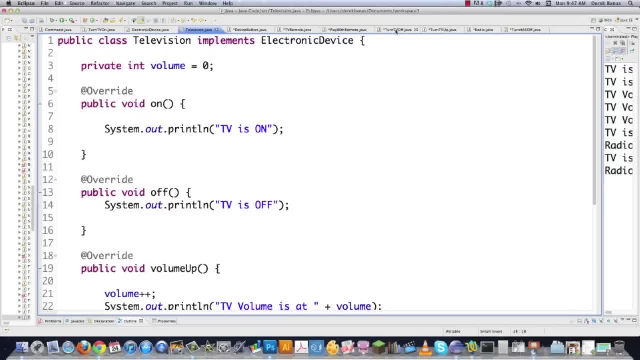 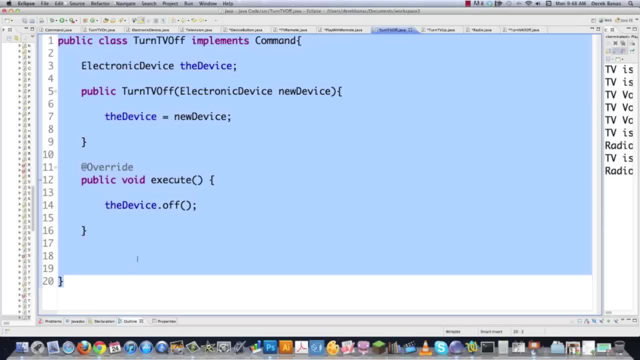 specific objects, So no big deal. So let's get back to turntvoffjava and look at it again. OK, And that's it, You're done. We just did that, As you can see, remember I said one of the negatives is it has a whole bunch of little. 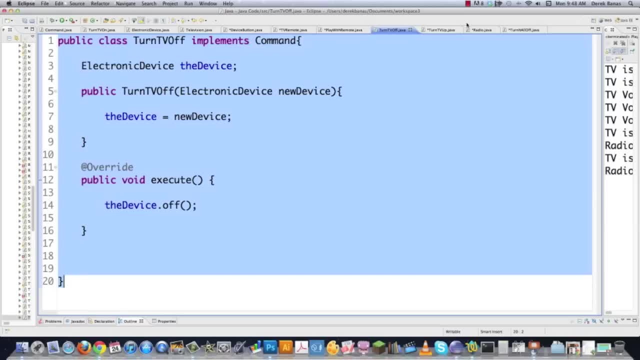 classes. Now that can also be a positive. So let's file, save that And let's go over to turntvupjava. Paste that in there. Turntv up Going to implement command just like before. Change that to up. Everything else is the same. 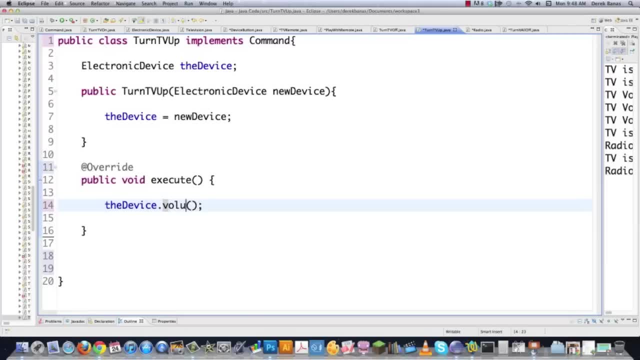 And then down here. we're just going to go to the device and we want to call the method volume up. There you are, Just did another one And if you want to, you can go and also create turntv down. But in this situation I'm not going to do that. 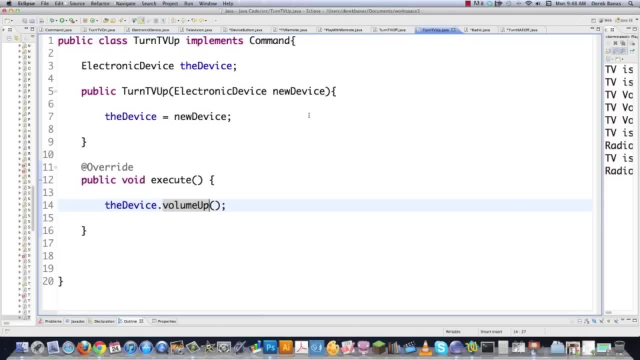 I'm going to show you in a minute how to use an undo command to do exactly that. So what does that leave us with? That leaves us with the invoker, And it is going to have a method. It's first off. its name is going to be device button, because we're using sort of like a 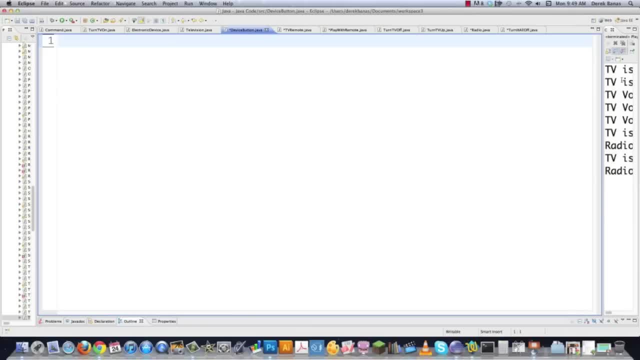 remote sort of thing here. So we're going to come inside of this and it's going to have a method called press that, when executed, is going to cause the execute method to be called, And then, of course, the execute method for the command interface then calls the method. 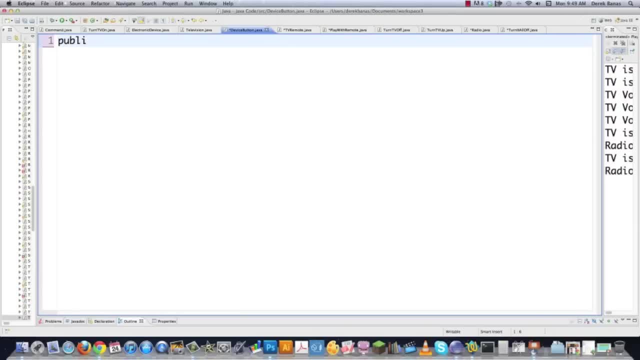 assigned in the class, And then it's going to pass the command interface, And then it's going to pass the command that implements the command interface. Okay, So just go public class- device button, There that is, And then it's going to be passed command, of course, in a generic sort of format. 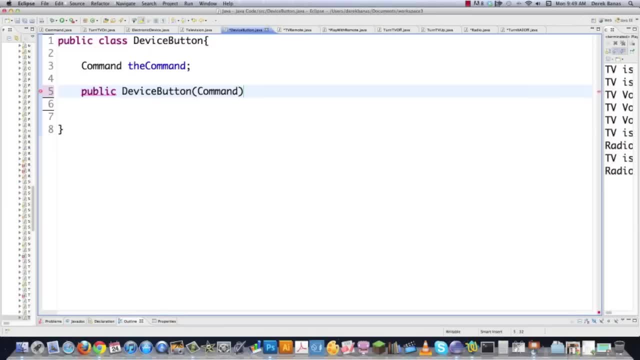 And we're going to go public device button command. New command is going to be passed over to it And I'm just going to go: the command, just like I always do, is equal to new command. And then we're going to create public press that I've been talking about. 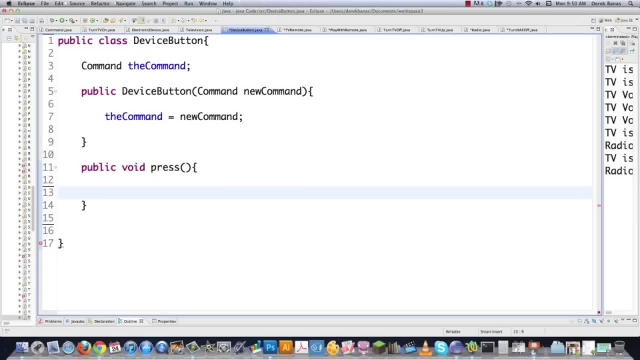 And now let's talk about the execute method. So now we've created a command that takes a function and says it's going to do something different. So the execute method is going to take a function and say, whatever the commands are, that the command is going to do. 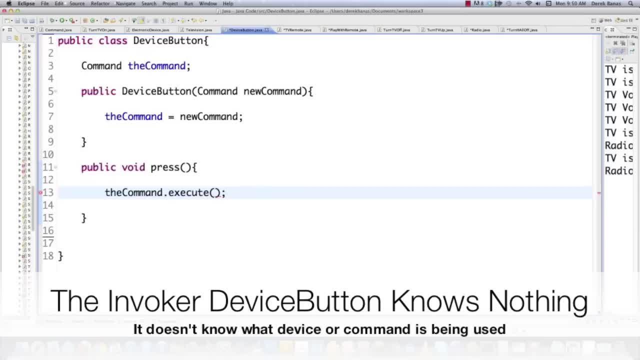 So an example of an execute method is going to say set command. So if I say set command, I want you to run, execute, Just like we said before, And then it's going to worry about command and all of the different objects that are. 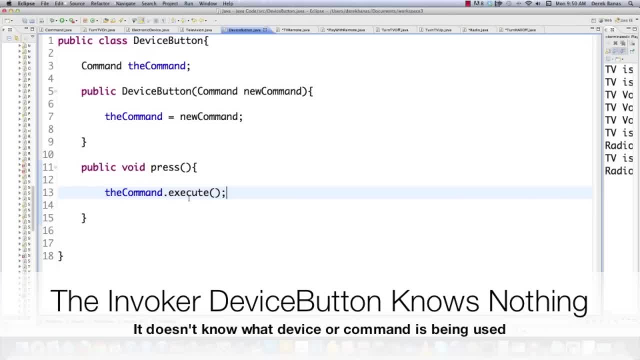 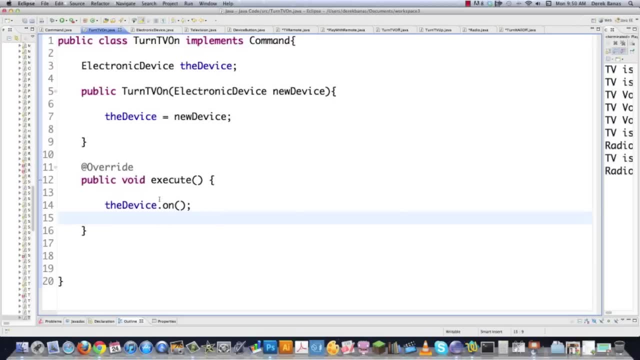 implementing the command interface are then going to just execute that execute command. Again, let's click on command. What's it do? Forces all commands to have an execute method. Here's turn TV on. There it does. Whenever execute is going to be called on this method, it instead calls another method. 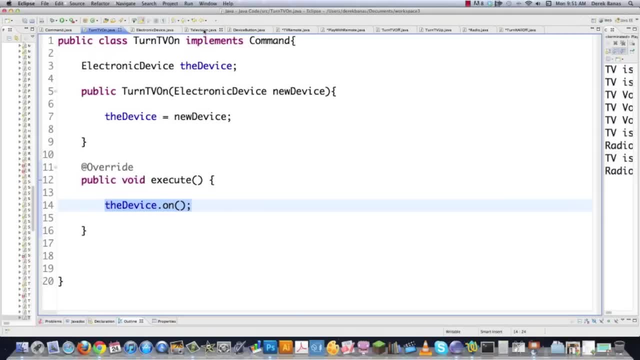 our device. And where is our device? Well, here's televisionjava. There it is. You just have to wrap your head around it. Just look at it from a couple different directions and you'll get it. So let's get back into device button. And yes, indeed, it's done as well. So then, what do we need to do? Well, 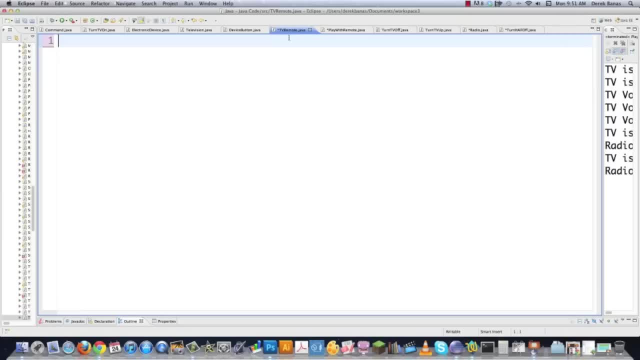 we're going to have to create something else called tvremotejava, And, in essence, what tvremotejava is going to do is it's going to return the type of device that we're going to use Now. I chose to keep this fairly simple, But of course you could have it work with multiple different devices. 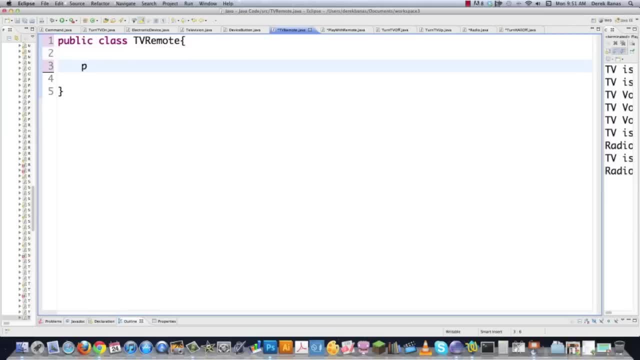 And I'm going to show you another way to work with a completely different device other than television here in a second. But basically what I'm going to do here is just go public static electronic device, get device. Okay, so it's going to have this static method inside of it. 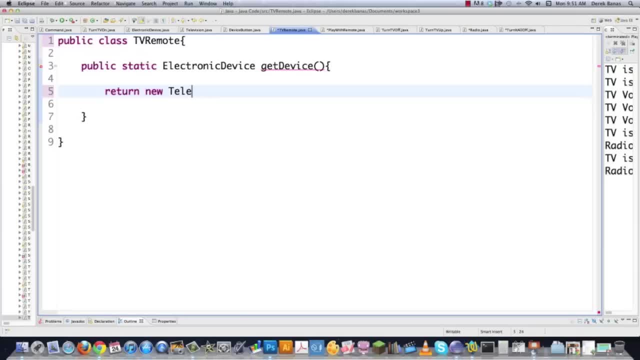 And in this situation, it's just going to return a new television which is just going to say: hey, we're just going to be using a television object here as our receiver to handle everything. So that's pretty simple. So now we're going to go into play with remotejava, And this is the 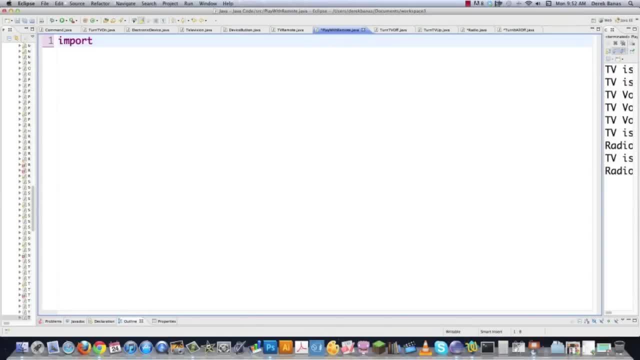 actual application And it's going to actually create all this stuff. So I need a couple different things here. I'm going to go Java util array list And then I'm also going to use a basic list. So just chop off the array part And there you go. Now you have all the libraries that we're 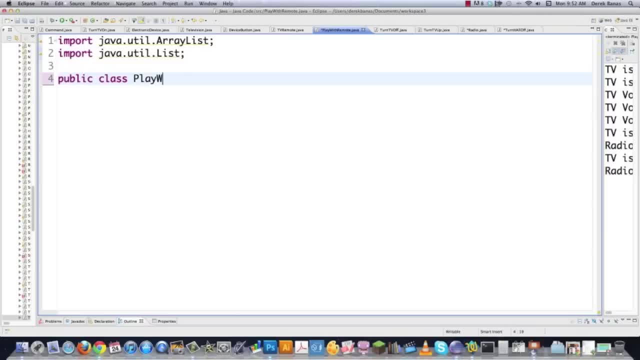 going to use here I'm going to go public class play with remote, And then what are we going to do? Since this is our application, we're going to have public static void main Args. Then we want to get the electronic device that we want to use And we're just going to go. 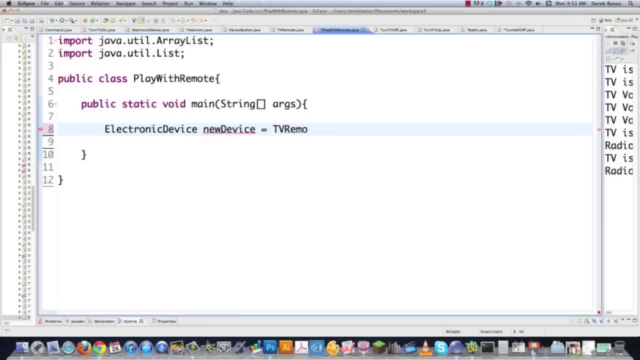 new device is equal to TV remote, dot get device. And what is that going to do for me? Let's just take a look, Here's TV remote. It's going to return a television. So it's going to say: hey, you want a device. Well, you're going to work with television. Now, of course, we could figure out. 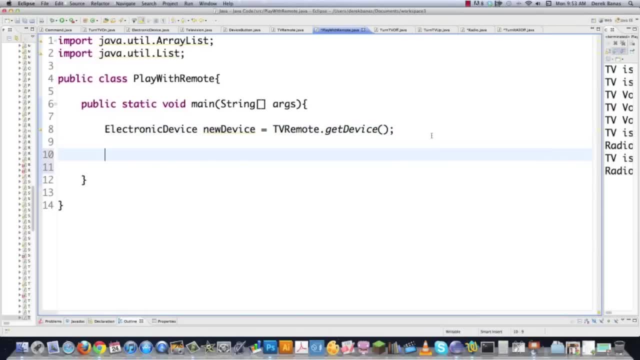 different ways to come in here and use all the other different devices, And in fact, I'm going to show you another different way to do that. And then what are we going to do? We're going to go turn TV on, And this is going to be called the on command is equal to new turn TV on. Here we are. 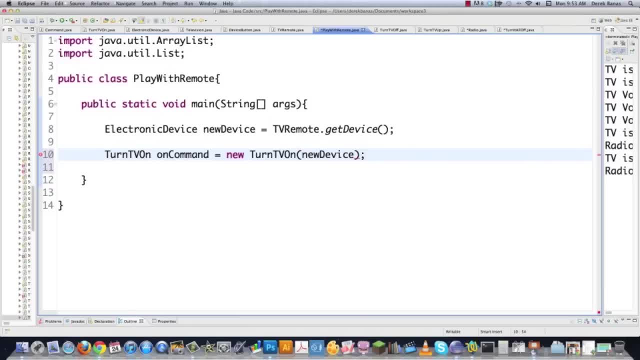 defining a command that we want this device to be performing. here We're going to send the device over and have it execute And, like I said before, turn TV on is just going to contain a command to turn on the TV when execute is called on this command object And then, of course, it's going 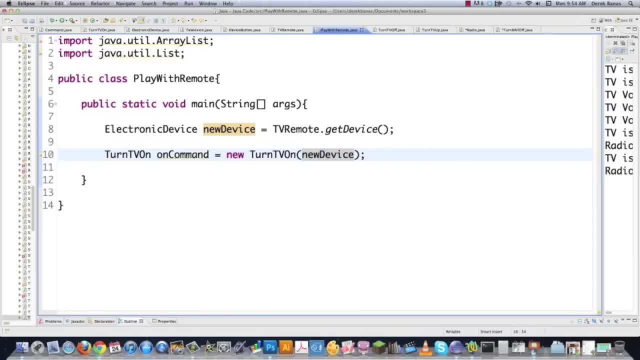 to execute the method on inside of the television device. Just let the information wash over you, OK, So then we're going to go device button. This is going to be the receiver And it is going to perform certain actions whenever it is called. So we're going to go to device button And we're 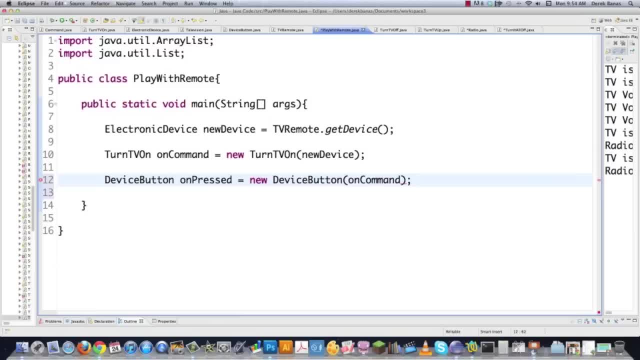 going to send it the on command Now. of course it just sees it as a regular command, But the receiver later on will figure it all out and make everything work beautifully. OK, So we have everything set up. We have our button which is going to set everything into motion. We have our 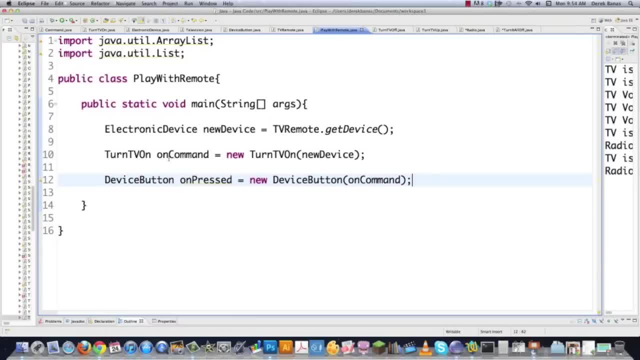 electronics device. It's going to contain all the methods we want executed, And then we have our device button. And then we have our device button. It's going to send a generic command over. that's going to be on command. The button is going to be pressed on. pressed. There we are Just. 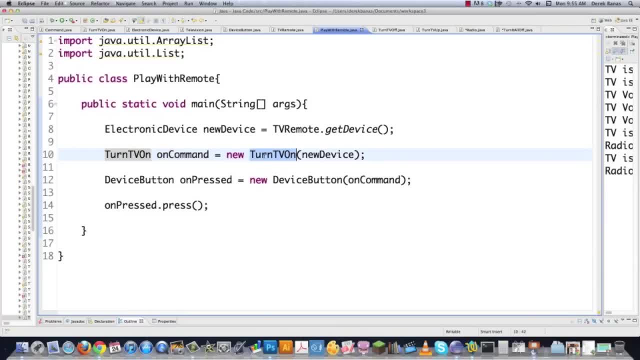 press the button on our remote control, Then what it's going to do is it's going to send a generic command over that's going to be on command that isn't really going to be generic because it's going to be called turn TV on, which isn't really going to be generic because it is of type turn TV. 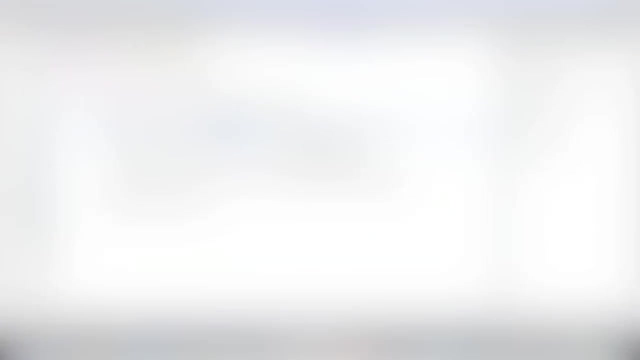 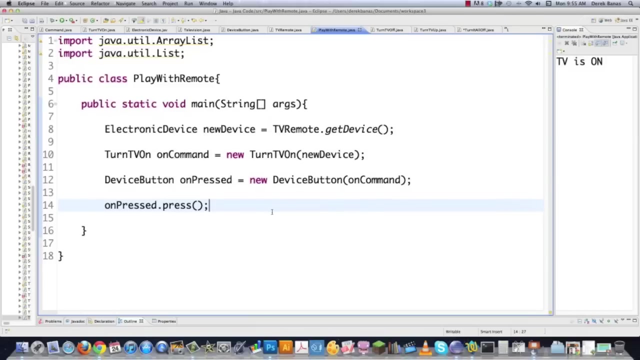 on, which, of course, you know, does one thing to devices: It calls the on method on them. So let's Sounds more complicated than it is. So how complicated is it to come in here and now turn our television off? Well, basically, we're just going to copy this and change a couple different things here. 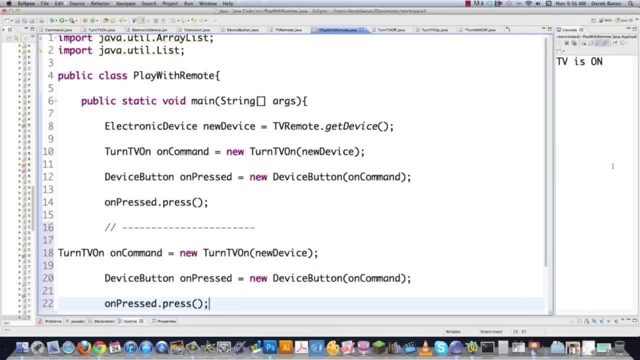 I'm just going to divide this up a little bit so it's easier to tell what's going on. I'm going to paste that inside of there. Now, if we want to perform a different action, what are we going to need to do? 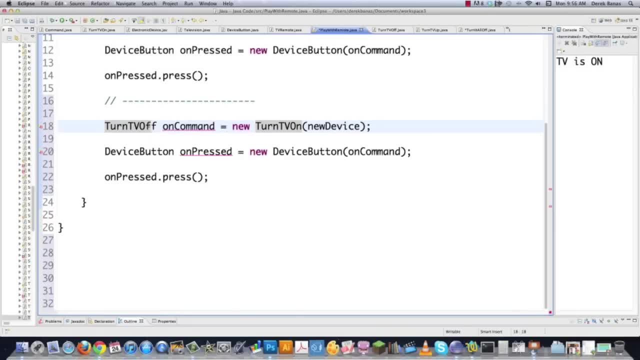 We're going to have to change the action that's performed. So now we're going to say turn TV off, and I'm going to call this guy the off command, And then, of course, we're going to need to change this to off as well. 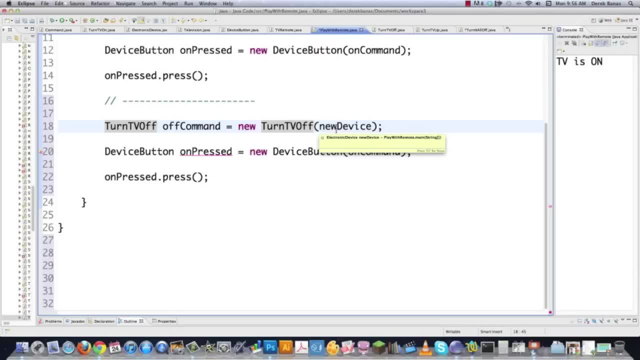 However, we're still going to pass the TV object, so that doesn't need to change. We're going to lop this off of here because we already defined it, And here we're going to pass the off command which we just created. 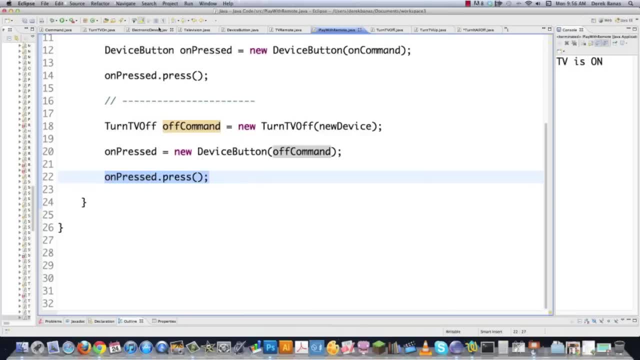 And here onPress doesn't care what type of command you're sending, It's going to work either way. So let's execute that. And you can see I turned the TV on and then I turned the television off. So let's see what happens whenever we come in here and start playing around with the volume. 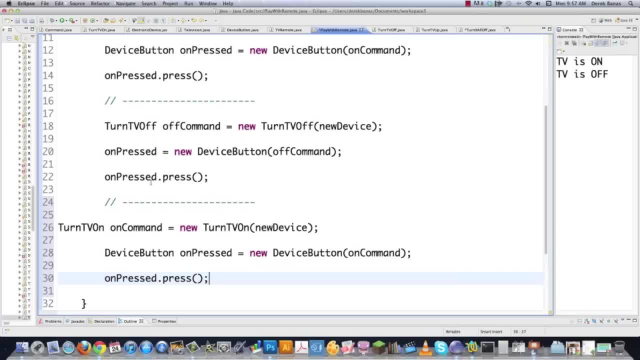 And even better, can we call Press multiple times without things flipping out? Yes, We can. Now, if we want to make the volume go up, we're going to go turn TV up. Just change our type on our command And then in here I'm going to go a volume up command: turn TV up. 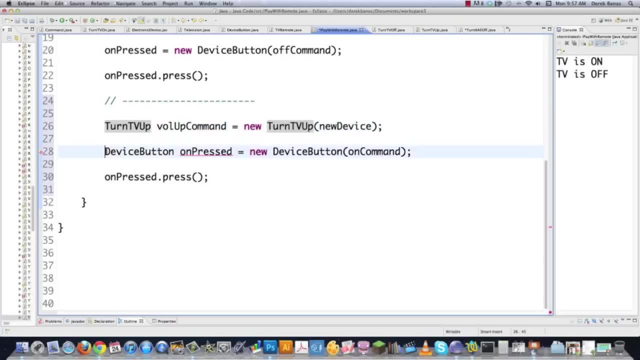 We're still going to use a generic device. Don't need to worry about that. OnPressed, of course, is going to change here, And then we're just going to send the right command to it like that, And then we're going to not only press the button once. 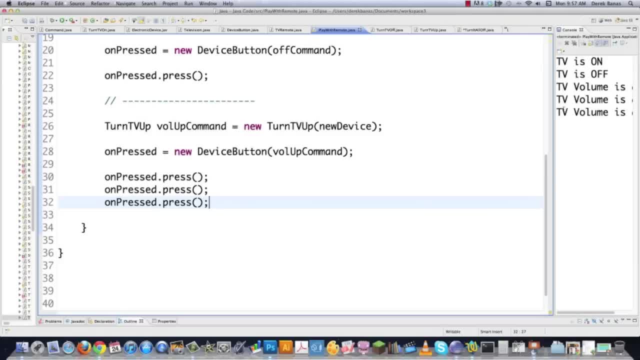 Why don't we press it a couple times and execute? And there you go, The volume: It's been increased. See One, two, three. It started out at zero. So pretty cool, Really, implementing a remote control here. So now let's throw another device into the mix, just to show you how simple that is to work with. 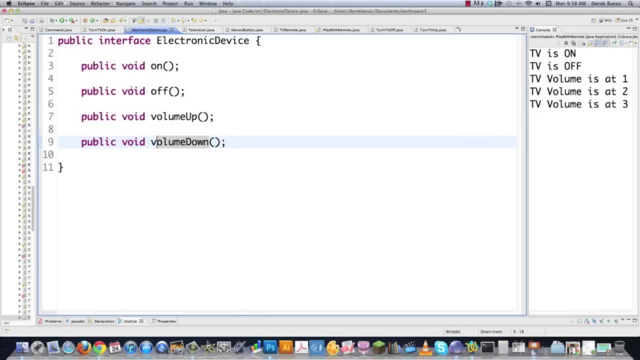 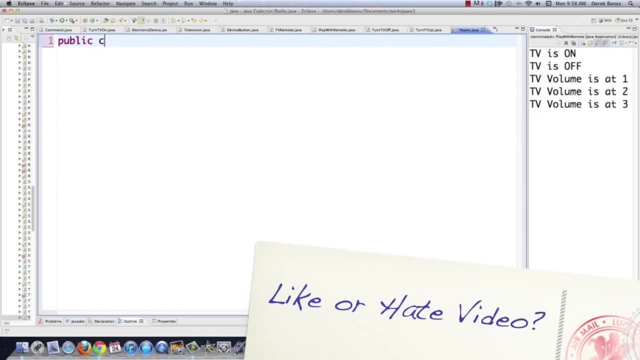 We don't have to touch electronic device in any way as long as we don't need to have any other methods implemented. Let's say we want to have radiojava created. How hard is that? Well, we're going to go public class: radio implements electronic device. 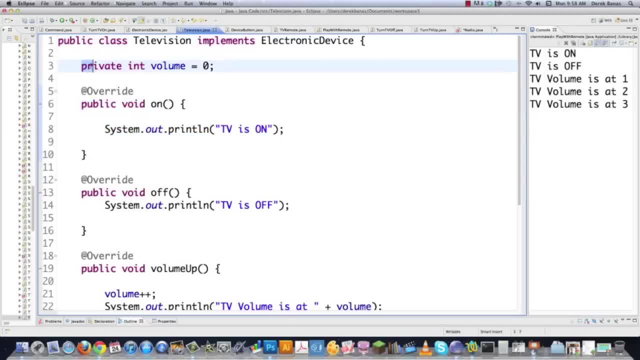 And just to save ourselves some time, I'm going to jump inside of here and I'm going to say, OK, I need all this stuff, Copy, jump back into radio, paste. There you go, Because the radio is also going to have a volume. 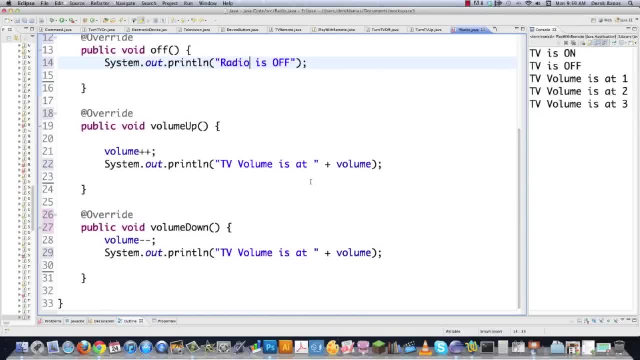 So now all we need to do is change this from TV to radio, and that's all we're going to need to do. Of course, you could do a lot more, but that works. And then we're also going to create the capability to turn off all the televisions and all the radios all at one time. 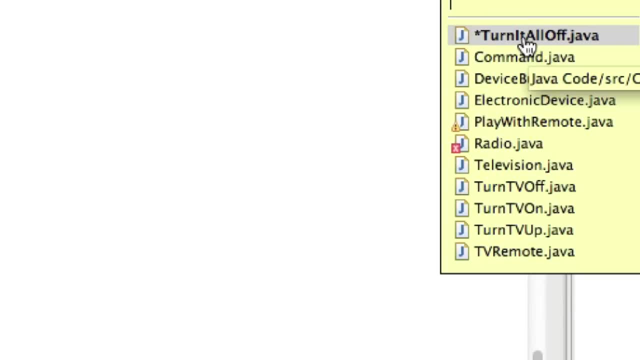 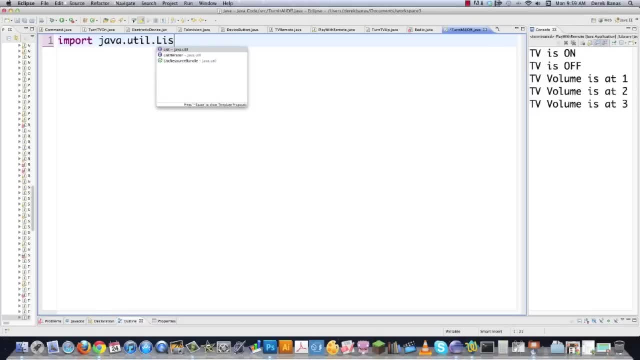 And to do that we're going to have a class called TurnItAllOffjava And to get that to work we're going to go Import Java Util and we're going to use a list to shut everything off. Public class TurnItAllOff. 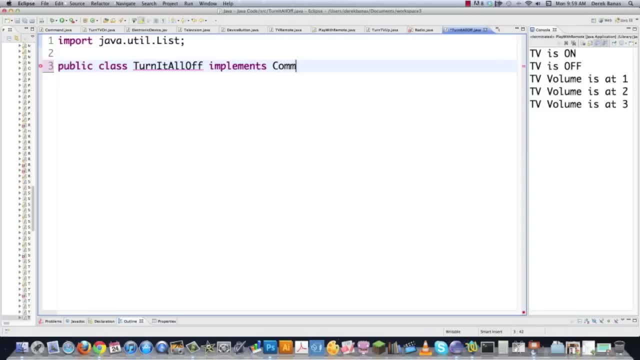 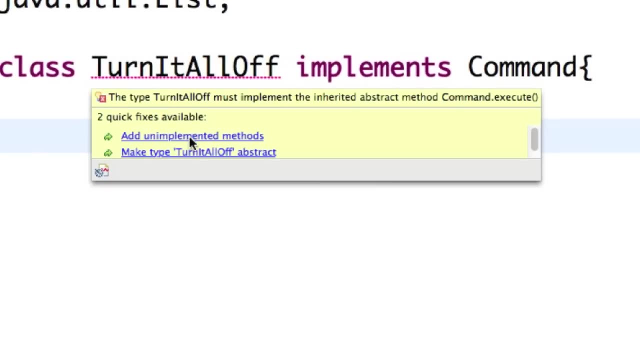 So this is like a master off switch to shut everything off at once, And this is going to implement the command again. And what is it going to force me to do? Pretty simple, It just wants me to implement execute, because everything that implements command must do that. 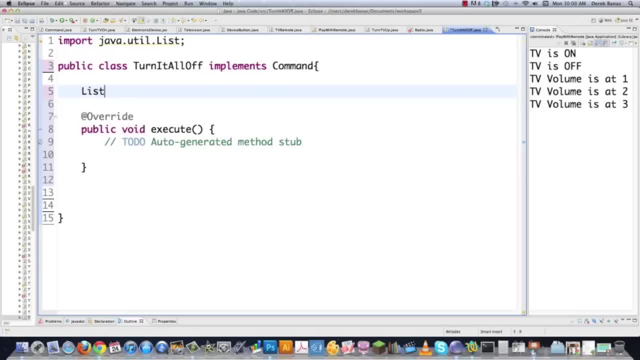 So what am I going to do here? Since I want to be able to turn all of them, All of them, off, I'm going to need all the electronic devices that are currently on or set up to work, with our little system sent to me as a list. 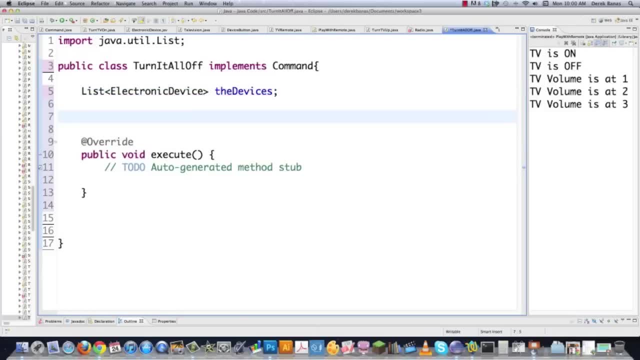 So I'm going to refer to those as the devices, just like that. Then I'm going to create a constructor public TurnItAllOff list And what's it going to be sent? Electronic device. So paste that inside of there. 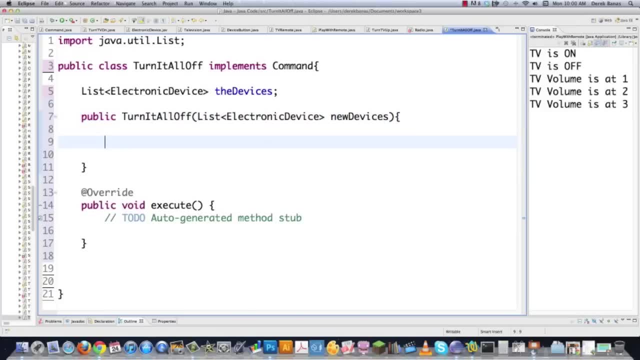 And here I'm going to say new devices like that, And then to transfer all of these devices, I'm going to control in one fell swoop. I'm going to take the new devices list that's going to be sent to me. 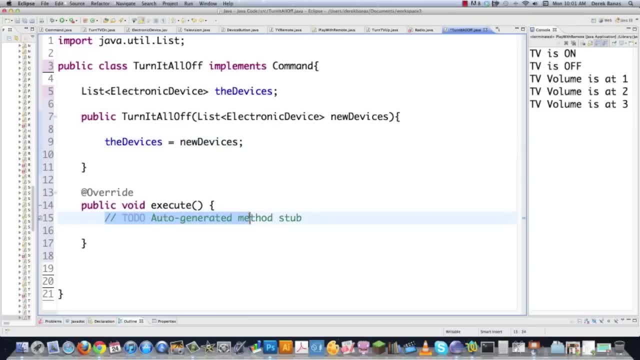 And I'm going to save it to my own personalized list. All right, Now we get to execute, And what we're going to do here with execute is we're going to shut all of them off using an enhanced for loop. So they are all electronic devices. 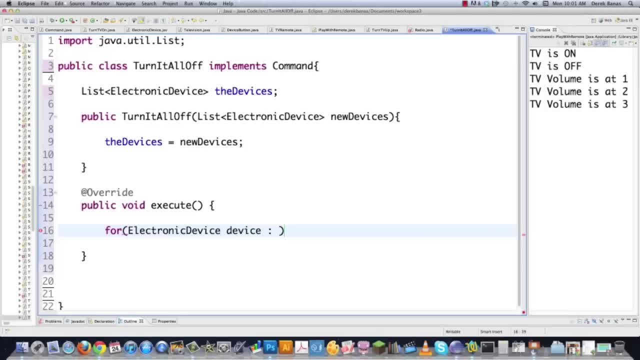 So that's cool, And we're going to say device individually, And then the devices of course is our list, And then to shut every one of these devices off, We just need to go. So device dot off. There you go. 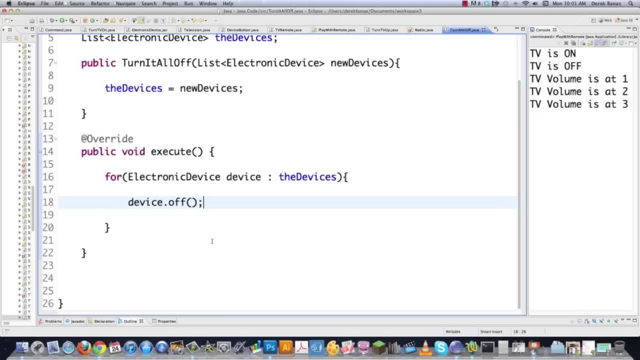 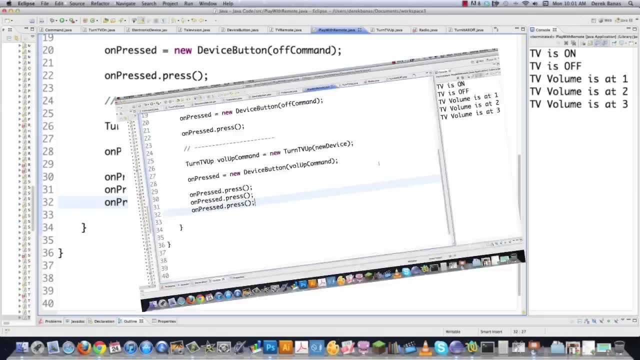 It's going to flip through every single device in the list and shut every single one of them off. That's pretty cool. So let's jump back over into play with remote dot Java And let's add those capabilities, which is going to be pretty simple. 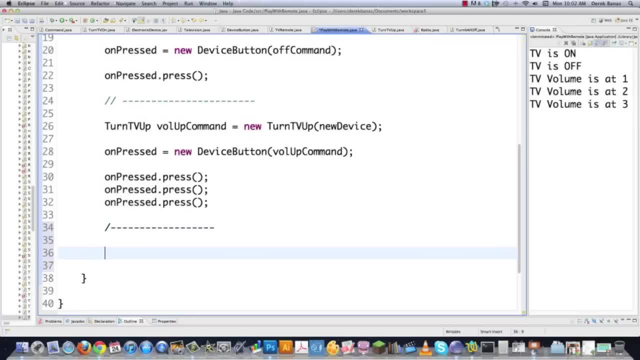 We're just going to come in here, make another dividing line inside of there so I can have a little bit more room, All right, So we need to create ourselves a whole bunch of different devices we want to work with. So I'm just going to go and create a new television and I'm just going to call it. the TV is equal to. 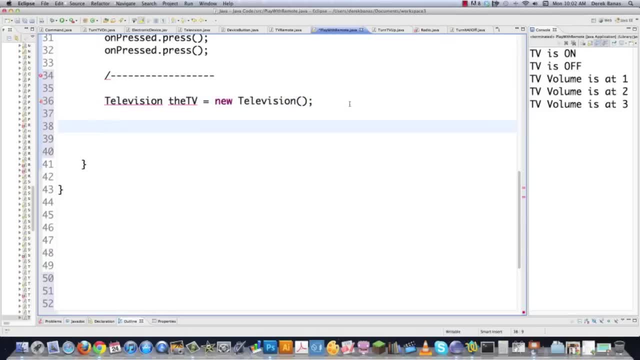 Television is a fun tutorial to do, and then I'm going to do radio. radio is equal to new and it is a radio object. Then I need to create myself a list and it's going to be electronic device. All devices is going to be loaded into it. 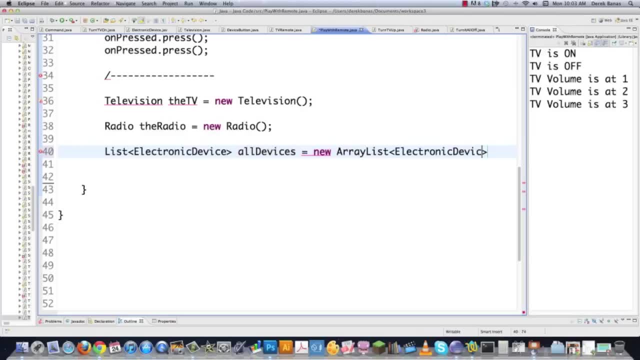 So I need to go new array list electronic device like that. Okay, So got that all set up. Now I just need to add my devices to all devices list and the TV- All devices- add the radio. got that set up And now what I need to do is just send the electronic devices to turn it all off. 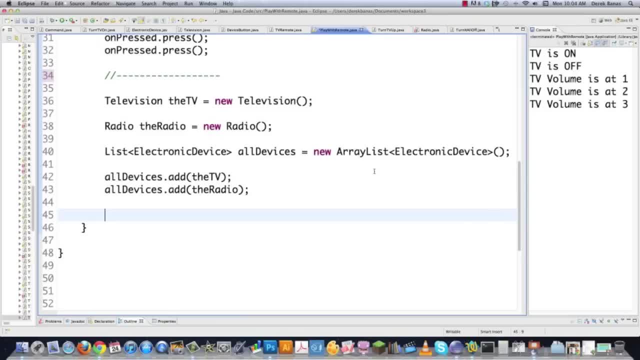 Where a call to run execute on this function will call off for each device in my list. Also pretty simple. So turn it all off. Turn off devices is equal to new. I don't feel like turn it all off again, So there it is. 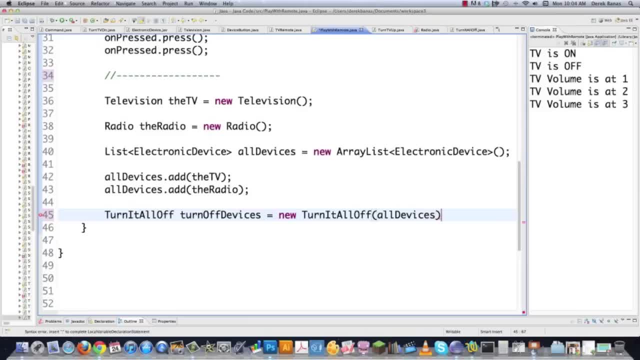 And I just need to tell it to shut off every single device in my list and it will. And then I need to go Device button. Turn them off is equal to new and then this is going to be device button. So it's like I'm putting a new button on my remote control dynamically and then going to send over turn off devices to it so that it knows what devices to shut off. 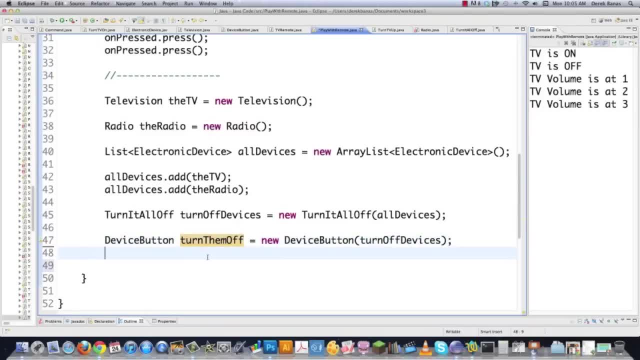 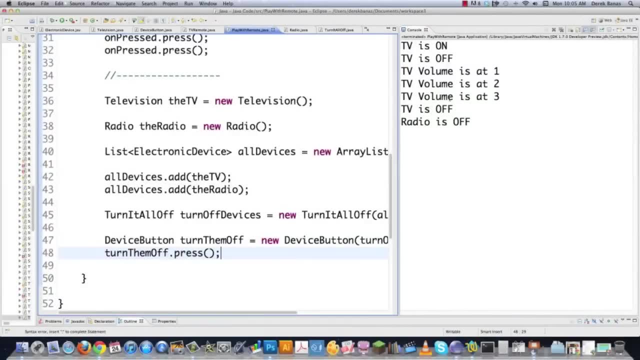 And now that I created my new button, I just need to call, press on it. to press that button and all the devices will be shut off. Let's execute it and watch it happen. There it is. So I turn the TV on, Turn it off. 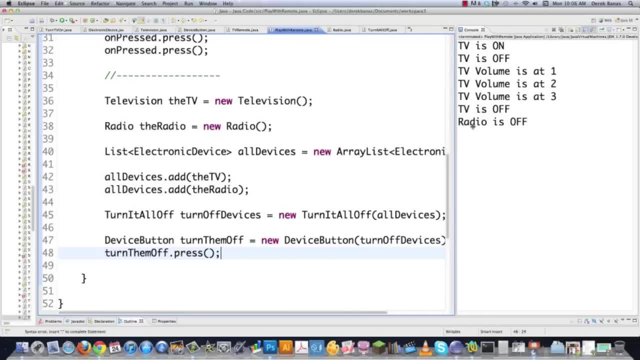 Turn the volume up to three, Turn The TV off and radio off, all in one fell swoop. So now let's implement our undo command. I'm going to do this to a certain extent and I'm going to leave part of it for you to do as homework. 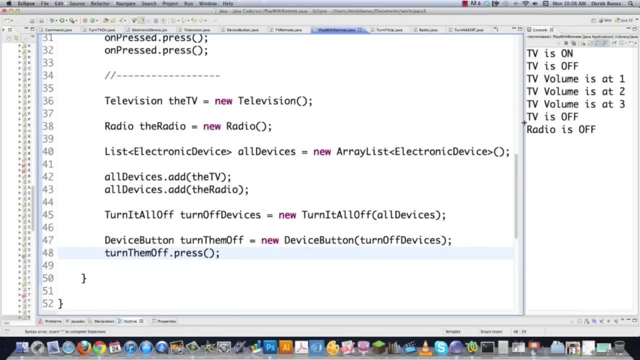 But either way, it is common to be able to undo commands using a command pattern. It's not required, but it's just something that is very common that you will see, And to do so the device button will have a method called undo, which will perform the opposite action or whatever the normal command performs. 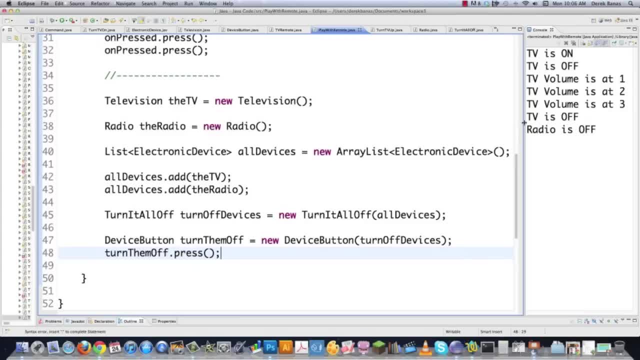 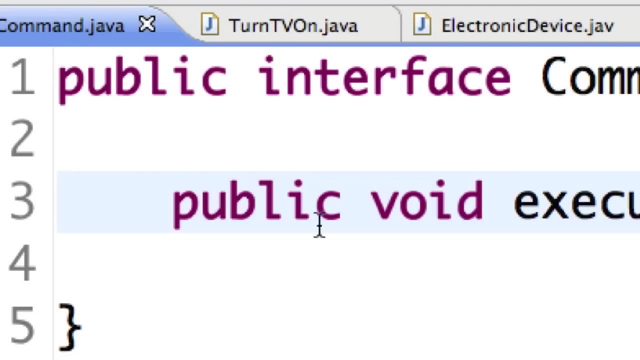 And to implement undo, you're just going to need to add it to every single class in which you have the execute method. So what are we going to need to do here? Well, we're going to have to go into command dot Java, which we created already, and we just need to implement the capability to undo commands. 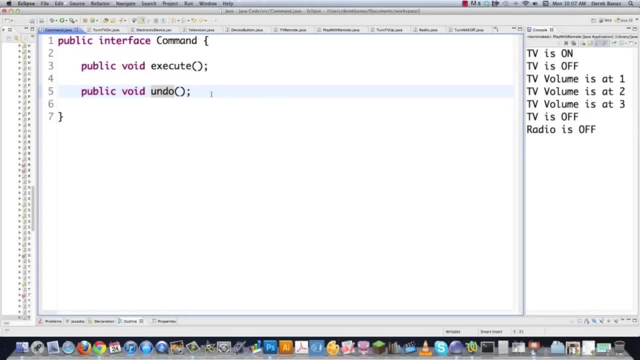 So I'm just going to change execute in this situation, Undo, file save. and there you go. Now you can undo commands. Now you're just going to have to go through all of your individual commands and also implement undo with those commands. So turn it off. 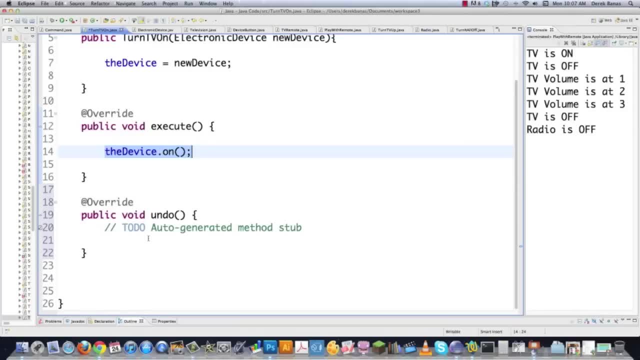 Now, all of a sudden, is going to say: hey, guess what you need to do undo now. So real simple. I'm just going to come up here. And what is the opposite of turning a device on? Well, of course it's turning device off. 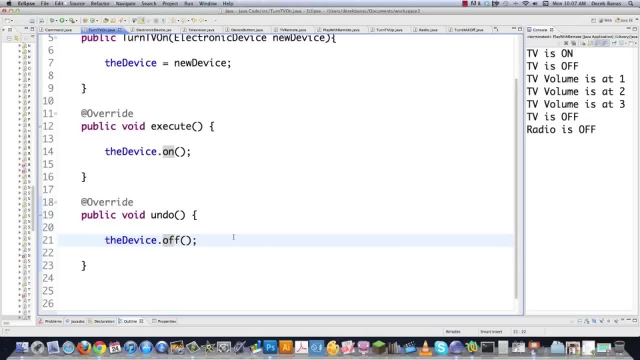 And look at that, You just did it. You just implemented undo in what? three or four keystrokes. That's pretty cool. I'm actually just going to copy this guy right here and then I'm just going to go into all the other different things here. 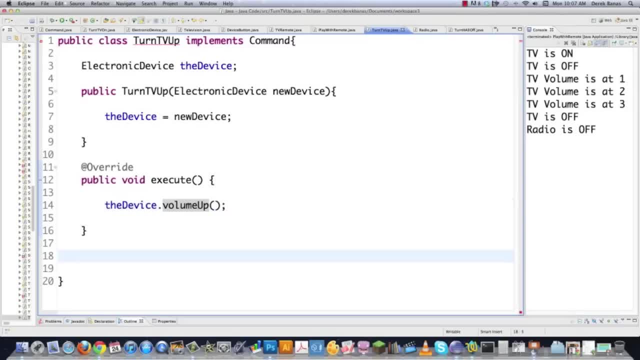 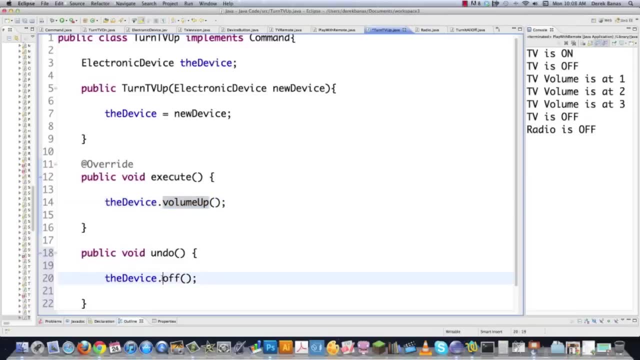 So turn TV up, Let's go into there and let's bounce down here, Paste that inside of there. And what is the opposite of turn TV up? Well, turn our volume down, Volume down, And there you are, Just implemented that. 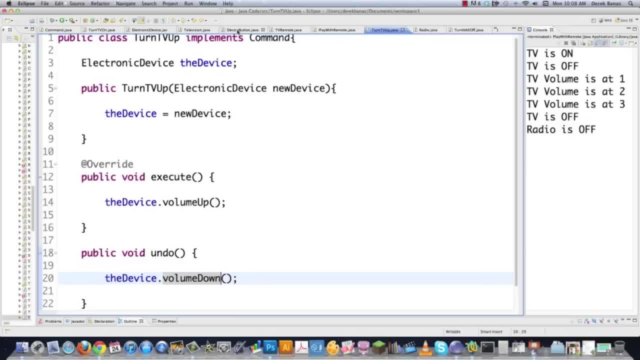 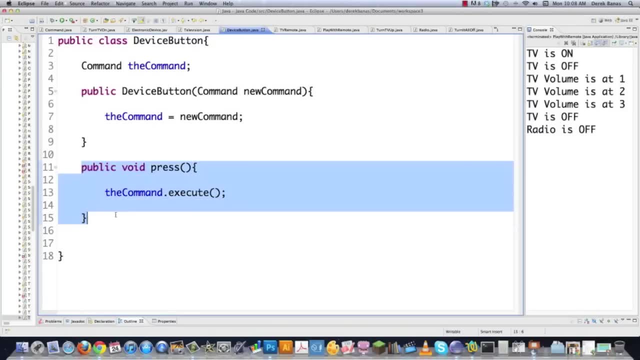 Not too hard. And then we also need to go into device button dot Java, because we're going to add ourselves a new type of button here And it's going to be a simple button. We're just going to copy, press And instead we're going to say: want to give them the capability to press undo. 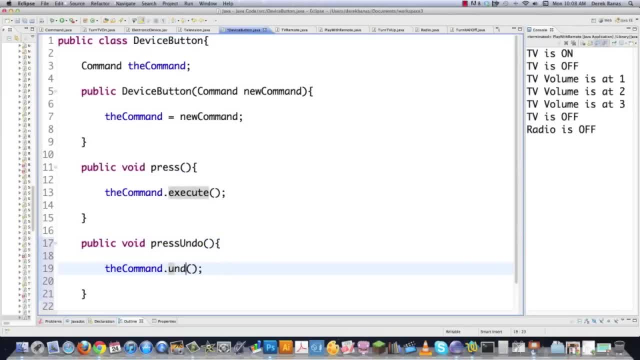 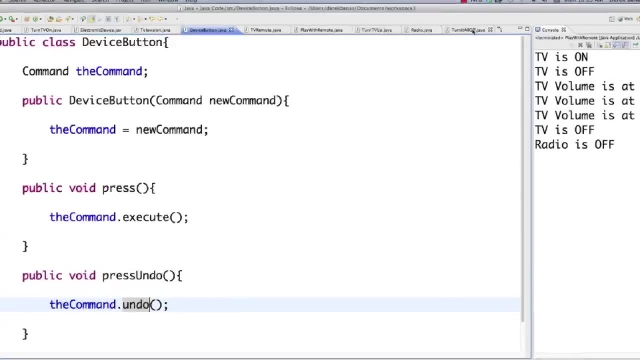 So there we are, And then the command here is going to be changed to undo, which we already created in our command interface. So also pretty easy. I could then go into turn it off. Where is turn it all off? There it is. 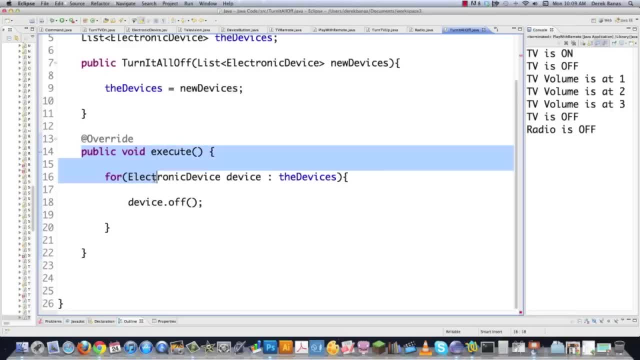 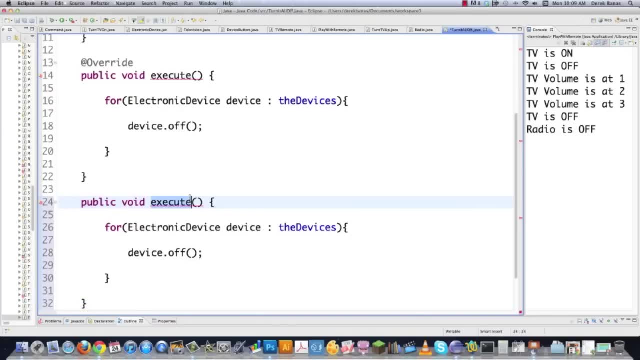 Turn it all off, dot Java, Bounce inside of there And pretty much do exactly the same thing that execute does, except we're going to do it using undo instead of execute. So tab and undo, And instead of off, we're going to switch off to on.